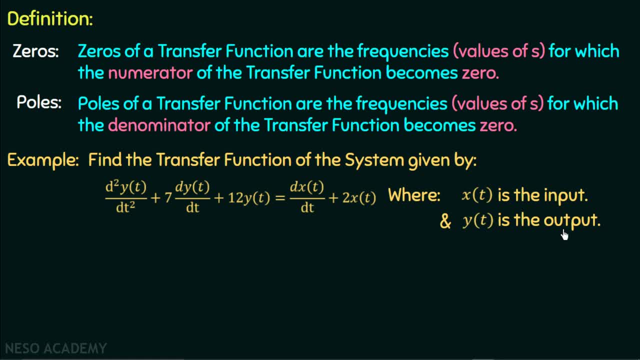 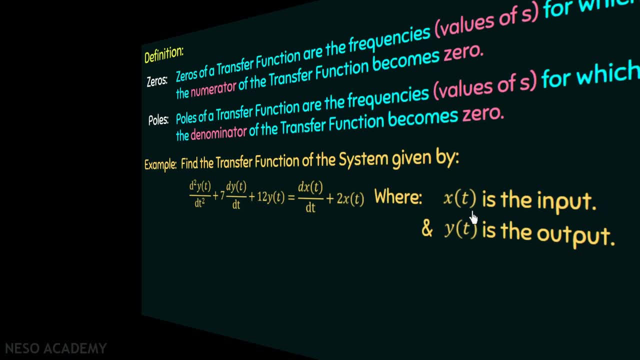 And we all know that the transfer function is the Laplace transform of output to the Laplace transform of input, by keeping all the initial conditions equal to zero. So, moving on to the solution, the first step is to find out the Laplace transform for this. 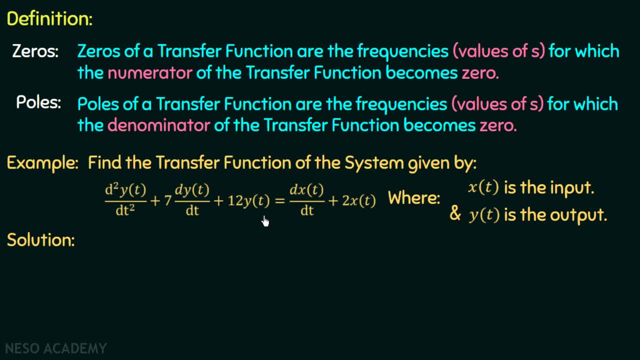 differential equation. So if we find out the Laplace transform and if we put all the initial conditions equal to zero, then we will get s square ys plus 7s multiplied ys is equal to s? xs plus 2 multiplied xs. Now we have ys common on the left-hand side and 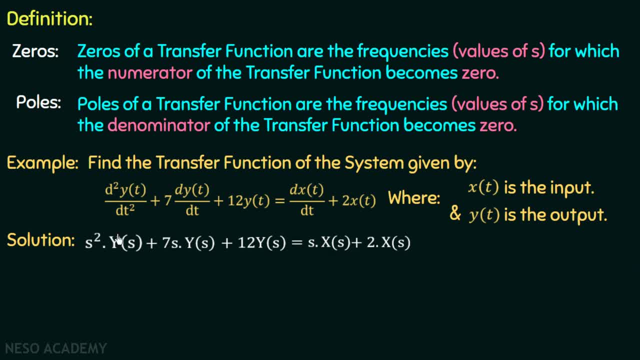 xs common on the right-hand side. So if we take ys common on the left-hand side, then we will get ys multiplied s square plus 7s plus 12.. And if we take xs common on the right-hand side, then we will get xs multiplied with s plus 2.. If we transpose xs on the left-hand 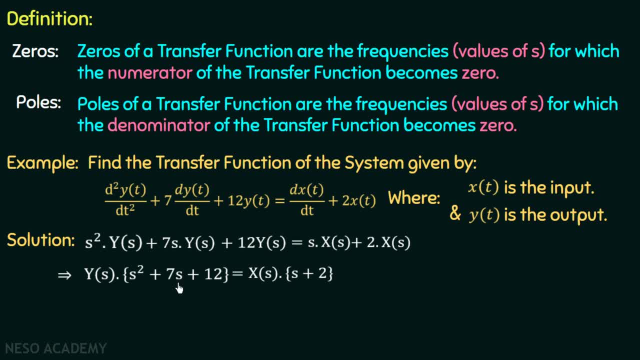 side. If we transpose this factor s square plus 7s plus 12 on the right-hand side, then we will get ys over xs is equal to s plus 2 divided by s square plus 7s plus 12.. If we factorize, 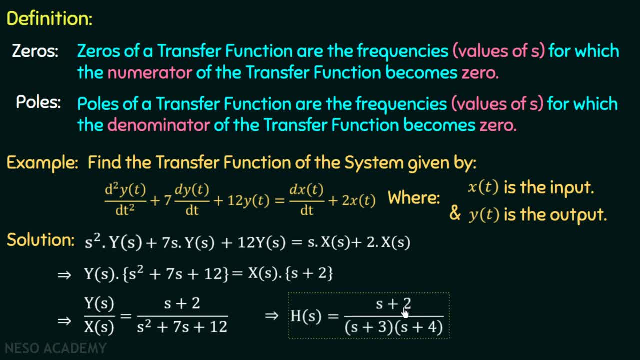 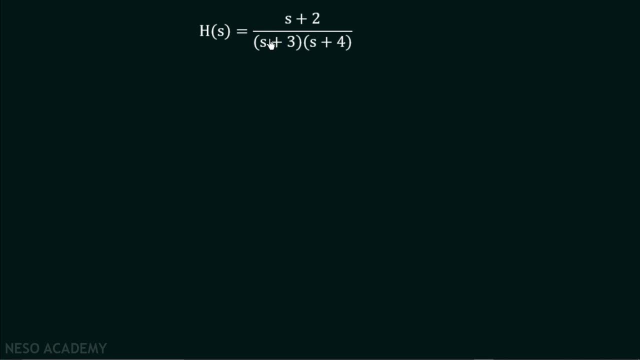 this term, then we will get the transfer function is equal to s plus 2 divided by s plus 3, multiplied with s plus 4.. And this is the transfer function for this system. So now we have our transfer function, which is to s plus 2 divided by s plus 3, multiplied with s plus 4.. Let us talk about zeros and poles, for. 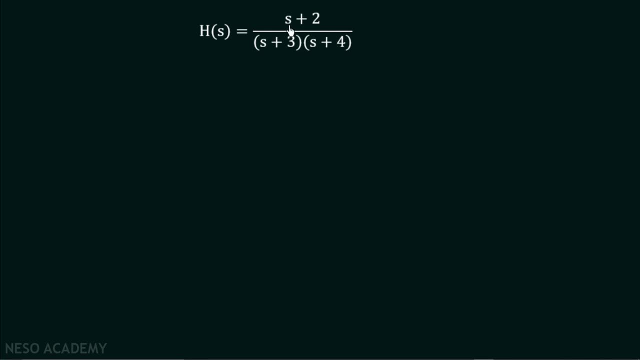 this transfer function. So we already know that zeros are the values of s, for which the numerator of the transfer function becomes 0. That means if we equate the numerator of transfer function equal to 0, then we will get the zeros of this transfer function And for this transfer function. 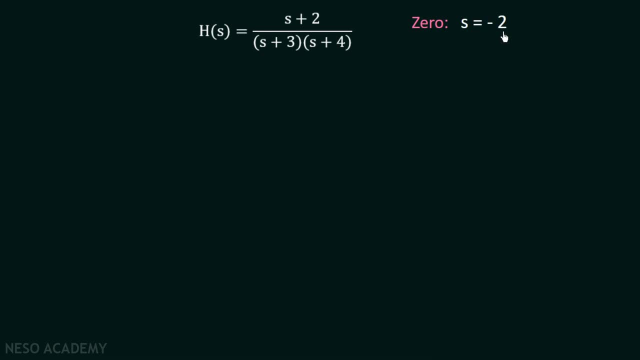 we have only one zero, which is s equal to minus 2.. So the zero for this transfer function we can say is equal to minus 2.. Similarly, if we talk about poles of this transfer function, then poles are the values of s, for which the denominator of transfer function becomes 0.. 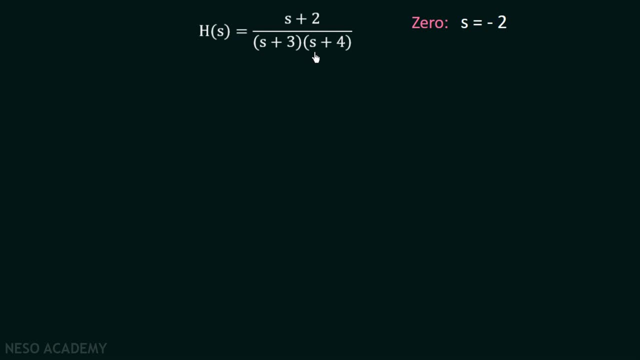 Or in the other words, the transfer function becomes infinite, because if the denominator is equal to 0, then the value of fraction becomes infinite. It means that if we equate 0 to 0, then the denominator of fraction becomes infinite. So if we equate the denominator of 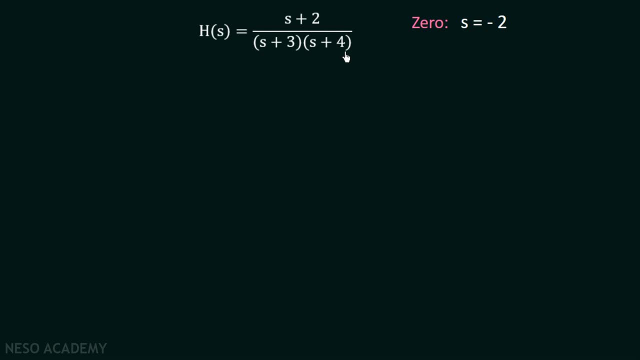 this denominator equal to 0, then we will have the poles of this transfer function: s equal to minus 3 and s equal to minus 4.. It means that there are two poles: minus 3 and minus 4.. So now we are. 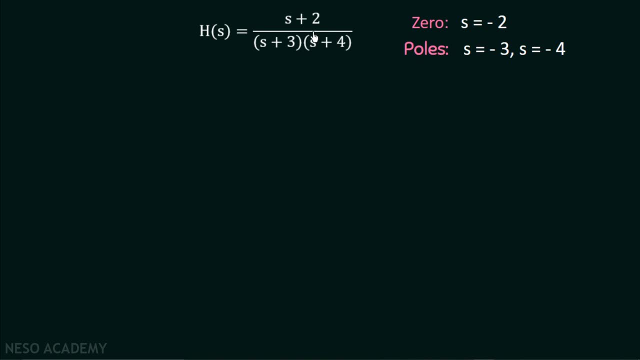 done finding the zeros and poles for this transfer function And if we want to plot these zeros and poles in the s plane, then we can plot it by using the pole zero diagram. The pole zero diagram is the plot on s plane which represents the locations of poles. 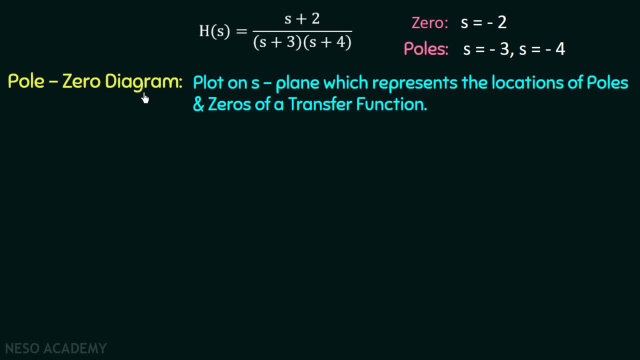 and zeros of a transfer function In a pole zero diagram, the poles are represented by a cross and the zeros are represented by a circle. So if we want to represent the poles and zeros of this transfer function on a pole zero diagram, then we will have this s plane, in which x-axis 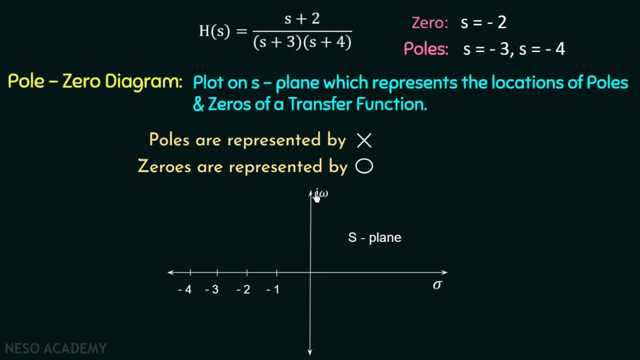 is the sigma-axis, which is the real part of s, and the y-axis is the j-omega-axis, which is the imaginary part of s. So we are having the zero 은s equal to minus 2, so we are having a circle 은s equal to minus 2, which will represent the. 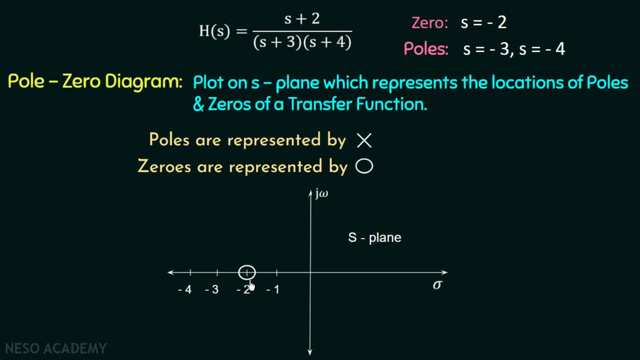 position of a zero at s equal to minus 2 for this transfer function. Similarly, we are having two poles, at s equal to minus 3 and at s equal to minus 4.. So we will have 1 cross at s equal to minus 3 and 1 cross at s equal to minus 4, and this is the pole zero diagram for the poles. 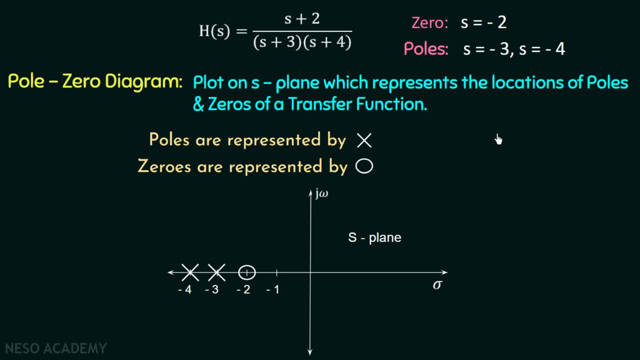 and zeros for this transfer function, and then Platzqualt, we see that we have coming to a third function. So now we are done with the introduction of zeros and poles for a transfer function, and we have also discussed the pole zero diagram by which we can represent the zeros and poles. 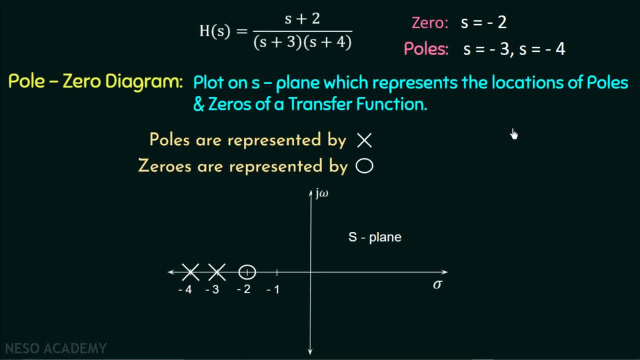 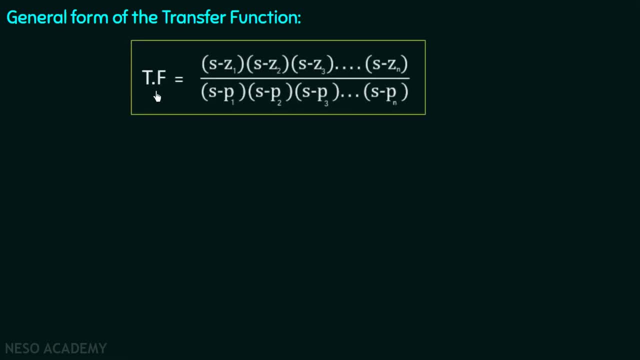 on an s plane. Now let us understand the zeros and poles for a general transfer function. So we are having a general form of transfer function which is given as transfer function equal to s minus z1 multiplied with s minus z2, multiplied with s minus z3, and so on, up to